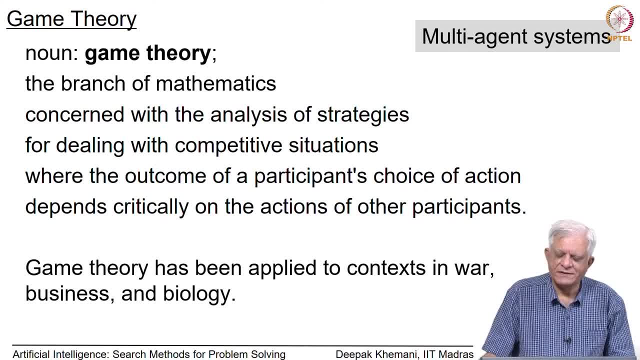 play or enter in any market. What are game theory? agents are rational and they act completely selfishly and to the best of their effort. essentially, AIM theory has been applied to various scenarios- economics, war, business, biology and so on- and it has been used to model such scenarios and try to study what should be the correct. 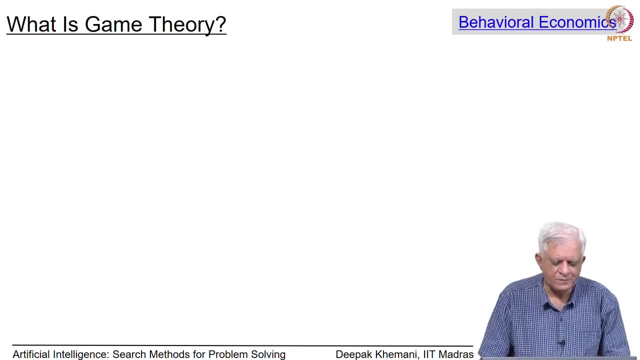 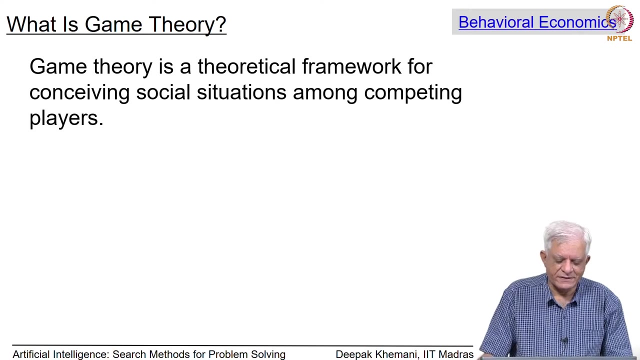 actions of agents in such scenarios. Here is another definition which we have got from this domain of behavioral economics: Game theory is a theoretical framework for conceiving social situations among competing players. essentially So, we are talking about how to model social situations where there are competing players. 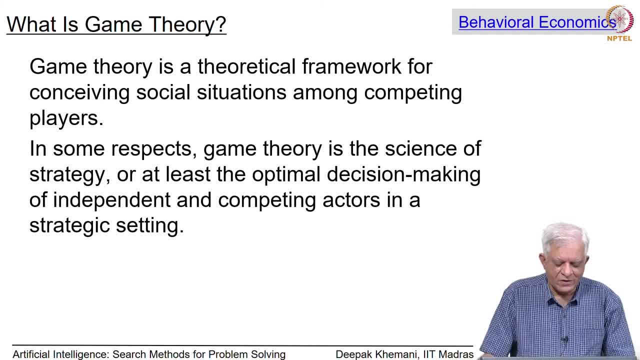 In some respects game theory is a science of strategy, or at least the optimal decision making of independent and competing actors in a strategy. So we try to figure out how, what are the kind of optimal decisions that that people make or players makes or agents make? in game theory terminology we often use the term player. 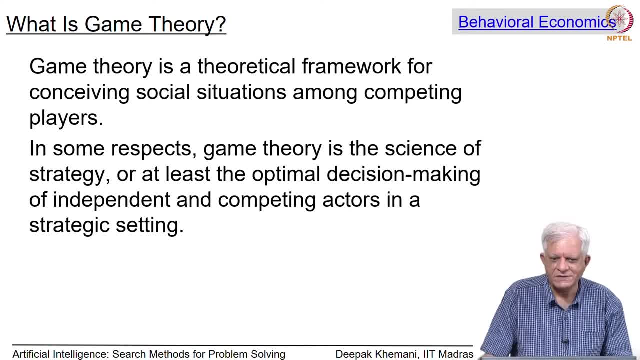 essentially, even though it may be a war like situation where we are considering game theory, it does not necessarily mean they are playing a game in that sense, but the terminology uses the term player. We can use the term player and agent interchangeably, So this is a good example. 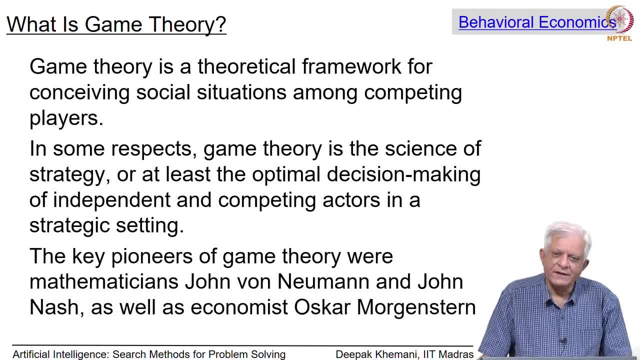 Thank you very much. Now game theory was I mean one credits John von Neumann who, amongst many other things that he did in his life, including giving us the stored program, computer model, sequential model for computing, He also is credited with originating this field of game theory, along with John Nash. 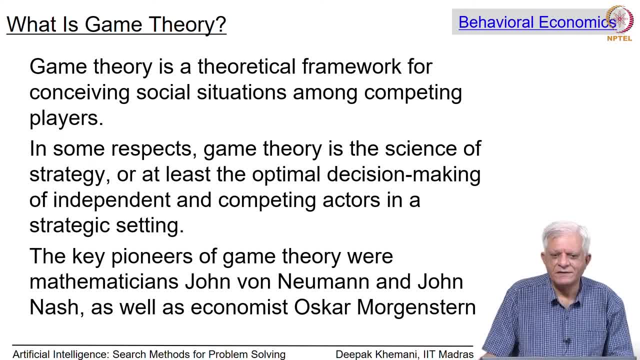 who you must have heard about, especially if you have seen that film called A Beautiful Mind, which is about John Nash and also the economist Oscar Morgenstern, essentially. So, as you can see, there are players from different communities which have kind of contributed to this field of game theory. 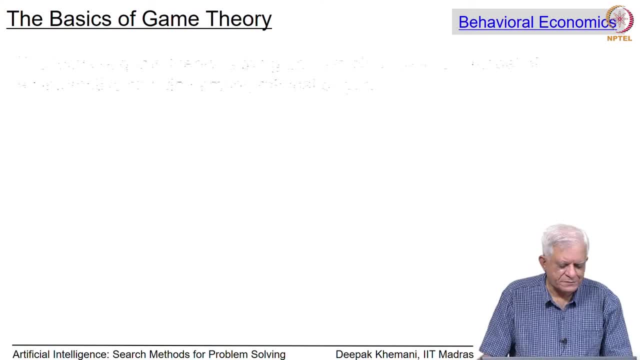 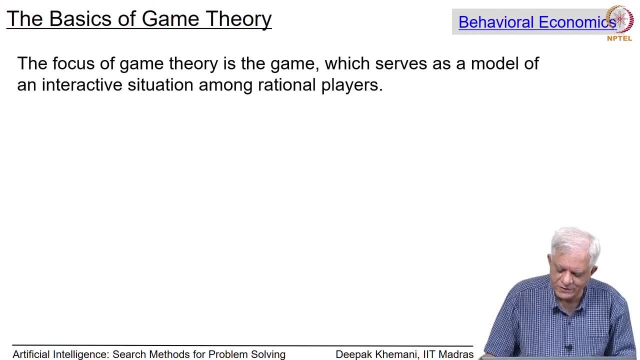 What are the basics of game theory? The focus of game theory is the game, which is the model of the social situation, scenario with in which this interactive situation where, amongst rational players- The key word here is rational players- The key to game theory is that one player's payoff 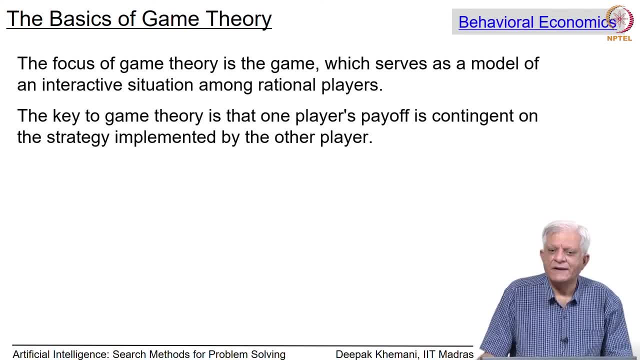 So we often use the term payoff. as to what do you get as a result of your choice Or as a result of your action? we use the term payoff. So the key is that one player's payoff is contingent on the strategy implemented by the other player. 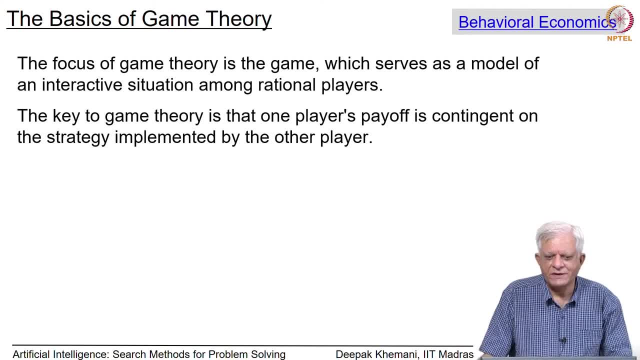 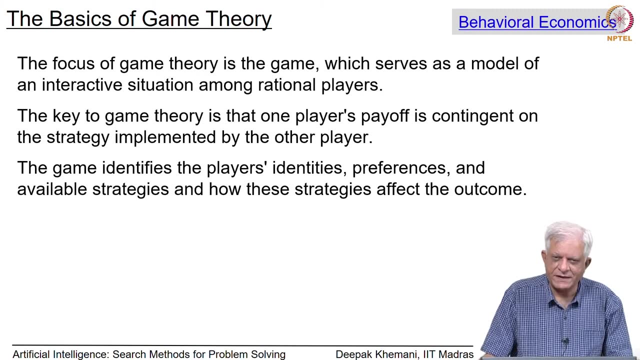 So, in game theory, we often use the term strategy, as to what is the plan behind your action or, as the term says, what is the strategy that you are using. The game, The modeling of the game, identifies the player's identity, The player's preferences. 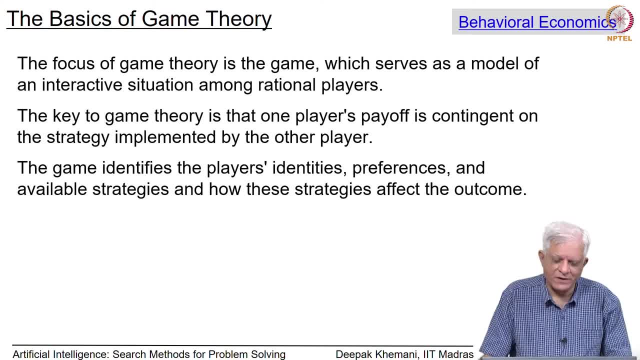 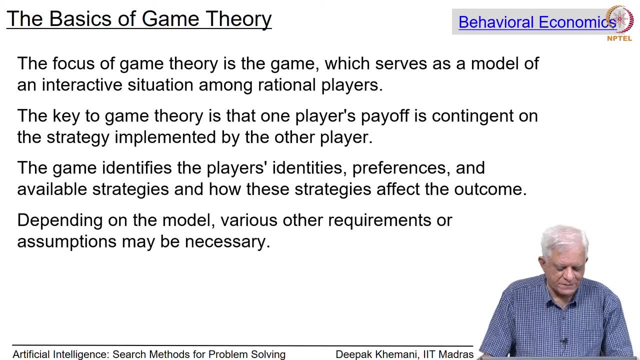 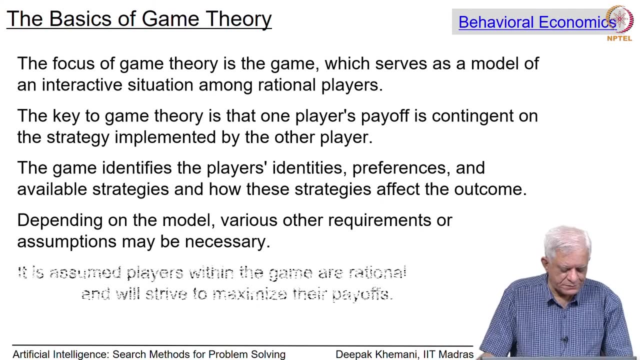 And available strategies and how these strategies affect their outcome. So all this we study in game theory. Depending upon the model, various other requirements or assumptions may be necessary, and we shall look at some classification of games as we go along. The key thing is that it is assumed that players within the game are rational. 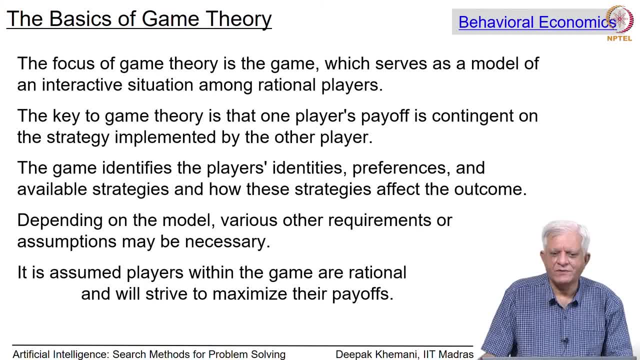 And will strive to maximize their payoffs. So if you know you are working or or the other participants are kind of making mistakes or acting foolishly or some such thing, we assume that everyone is rational and everyone is acting to maximize their own profits. in that sense they are selfish and we want to study. 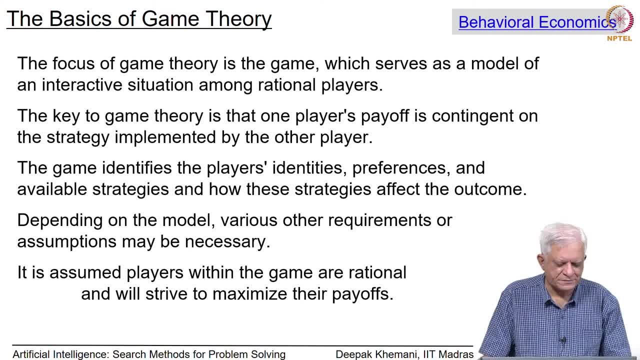 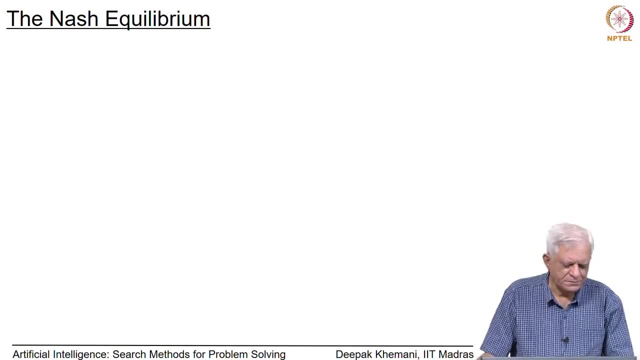 as to what can happen in such scenarios. essentially, Now, there is something called the Nash equilibrium, which is, as you can guess, named after John Nash, and it says that Nash equilibrium is an outcome. after all, the players have made their decisions, that is reached, which, once achieved, means that no player can increase. 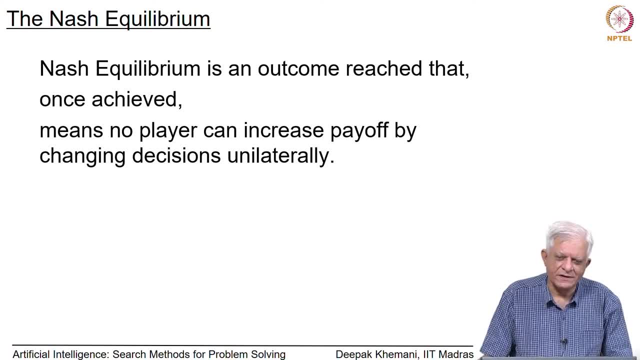 their payoff by changing the decisions unilaterally. So in some sense, Nash equilibrium is where the game will settle into, because if any player deviates from the choice that leads to the Nash equilibrium, They will actually decrease their payoff, or they will not increase their payoff, at least. 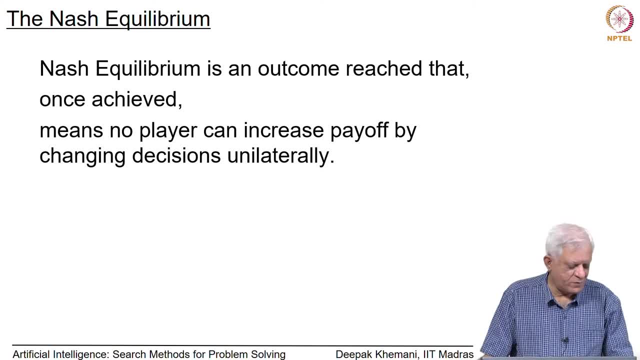 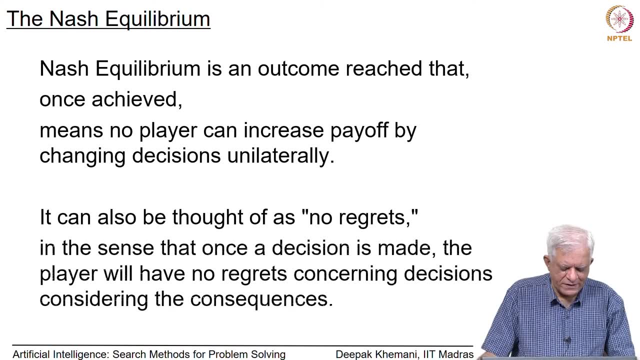 So it is an equilibrium where, once it is reached, no player can deviate from it. essentially, It can also be thought of as no regrets, in the sense that you have made a choice and once a decision is made, the player will have no regrets concerning decisions considering. 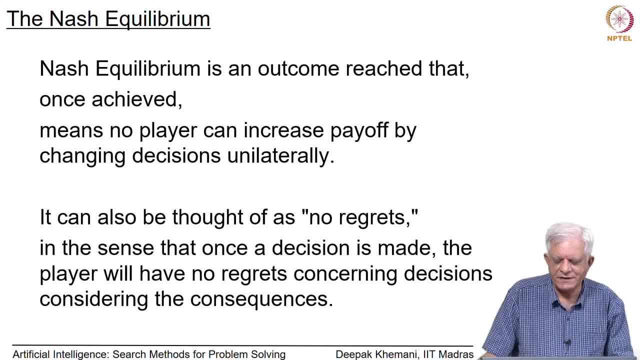 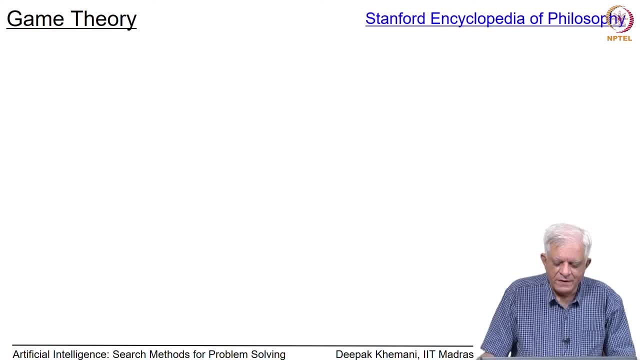 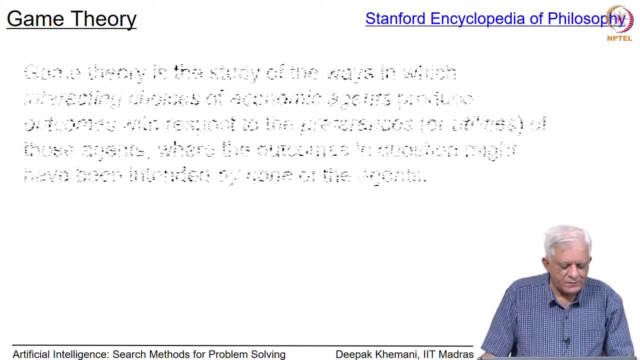 the consequences because the player knows, or in some sense the player believes, that he or she cannot do better, or it if it is a program. Here is another definition of game theory from the Stanford Encyclopedia of Philosophy: Game theory is a study of ways in which interacting choices of economic agents, So economic in 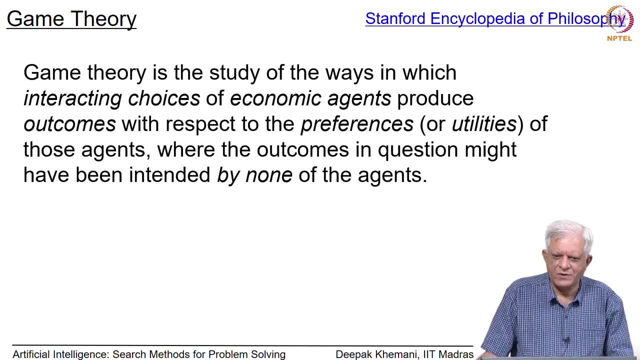 the sense that you are trying to maximize your payoff. So it is a study of ways in which interacting choices of economic agents produce outcomes with respect to the preferences or utilities. So we always assume that the agents have some goals or which we call as preferences, or we call them as utility. What do they get? 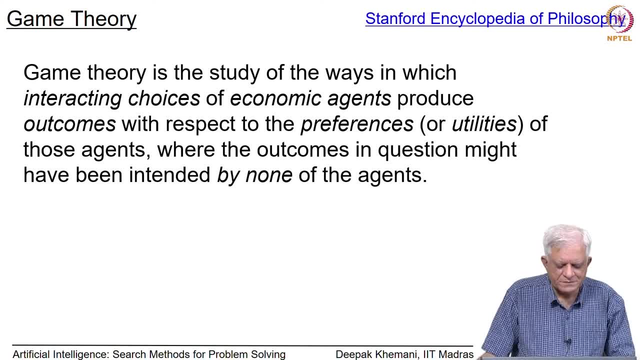 out of the game. So it is a study of ways in which interacting choices of economic agents produce outcomes with respect to the preference or utilities of those agents where the outcomes in question might have been intended by none of the agents. So it is not as if you are. 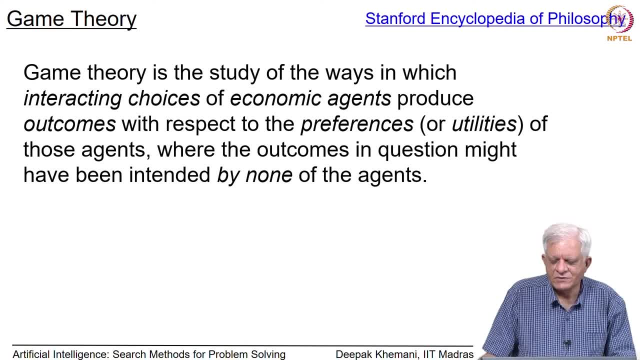 acting unilaterally and you are driving the whole social situation as a dictator, or it only depends upon your actions, It depends on other actions, and it may. the final outcome, the final Nash equilibrium, for example, could be something that you yourself had not intended. 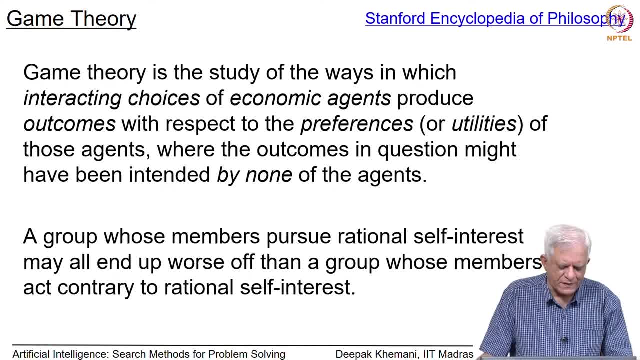 to be So. a group whose members pursue rational self-interest. So that is the assumption in game playing May all end up worse than others. Worse of then a group whose members act contrary to rational self-interest. So we will see. 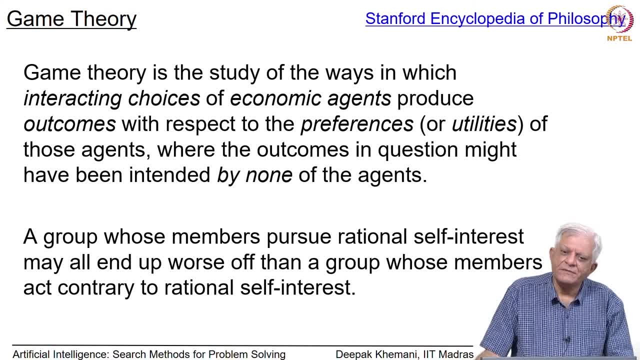 an example of this is that sometimes being totally selfish can end up. you can end up in a situation worse than you would be otherwise. A glaring example in today's world is our treatment of our earth. 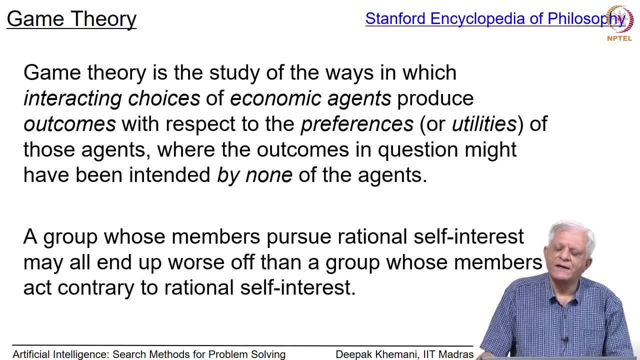 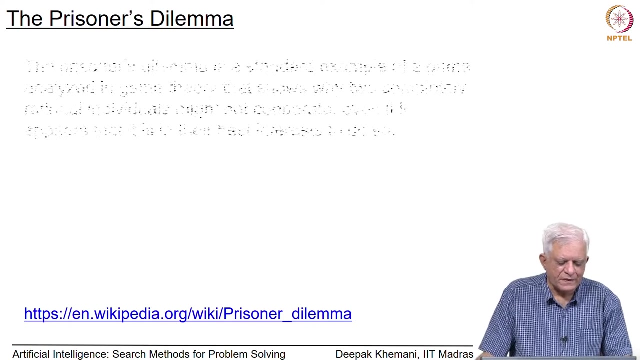 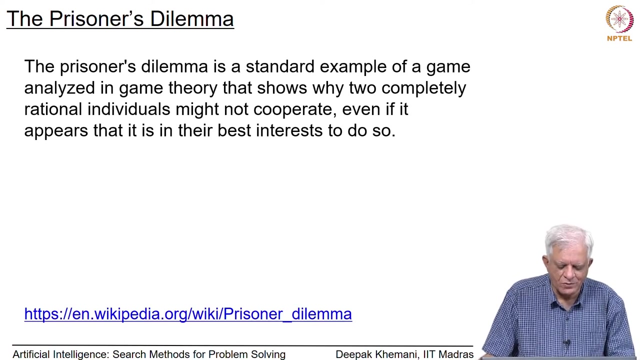 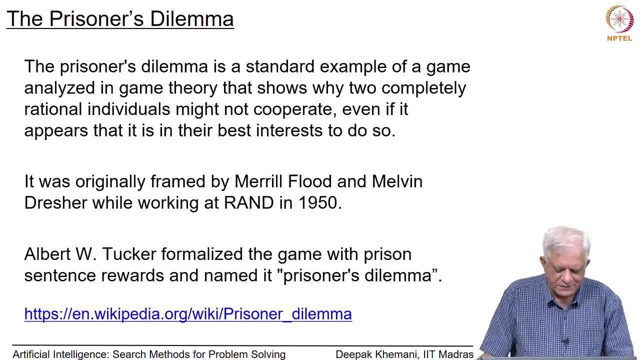 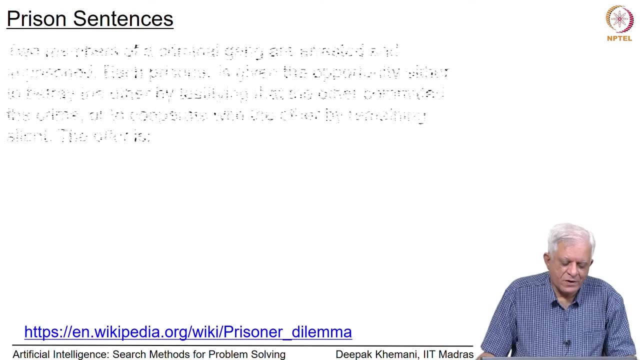 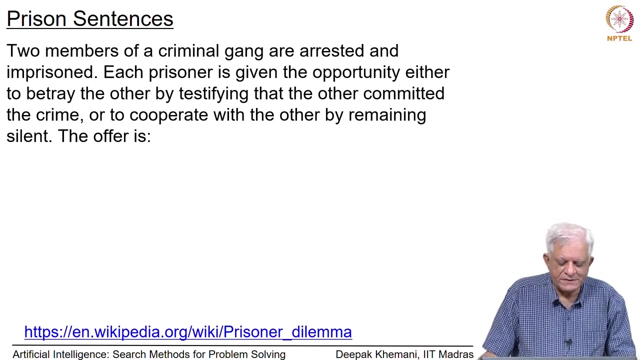 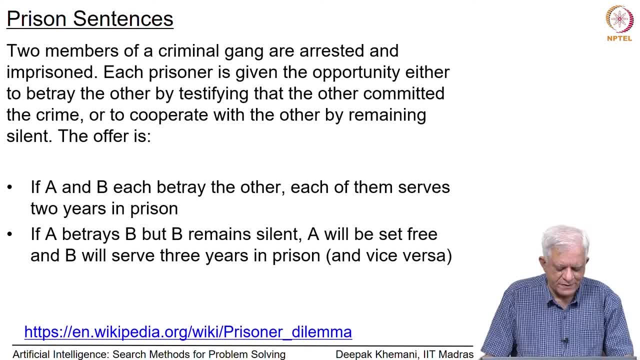 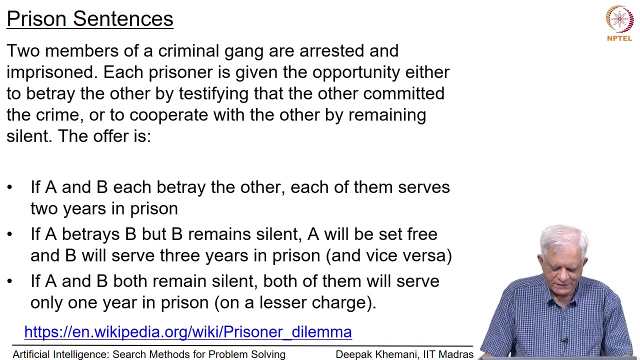 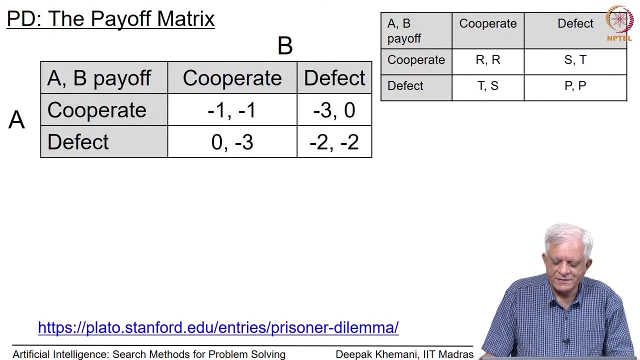 So we can now model this business dilemma as a table. it is a payoff matrix, and what you can see in the payoff matrix on the left hand side is the actual game that we are talking about. instead of betrayal, we have used that term, defect, which we got from the 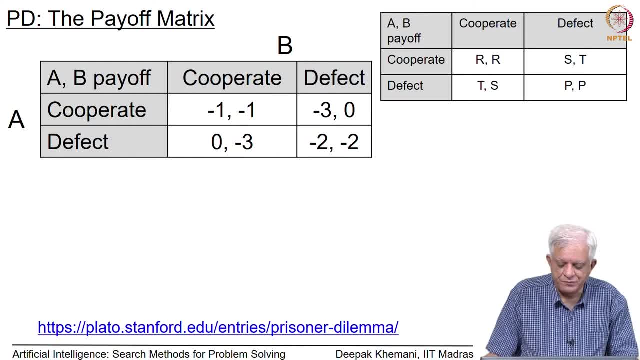 Stanford side and you can see that if both cooperate they get 1 year each on the lighter sentence on some some related charge, you know, like possessing a fire arm or something like that. If both betray each other, they get minus 2 each, minus 2 each. So the left hand side figure is for player A and the right hand side number is 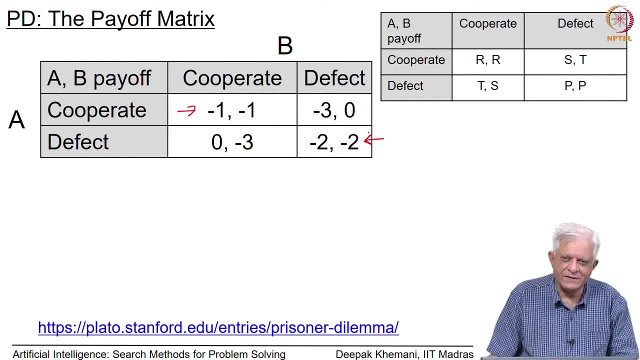 for player B, essentially, and the choices are given in the respective rows and columns. If A betrays B, then you can see that A gets off with 3, but B gets a prison sentence of 3 years, which we have modeled as minus 3 here, the payoff is minus 3.. And, conversely, if B 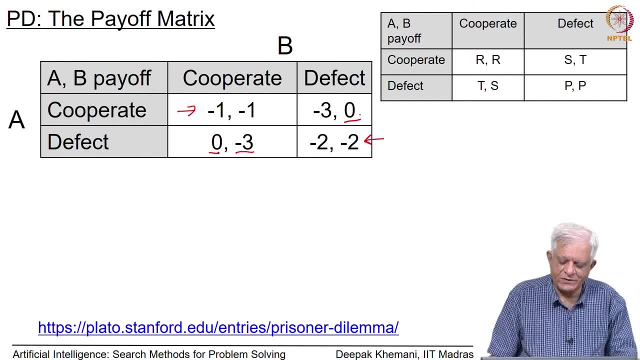 betrays A, B gets let off with 0 and A gets a prison sentence of minus 3.. So we can kind of model this, as you can see more generally In the payoff matrix on the right hand side and where you can see that either they can. 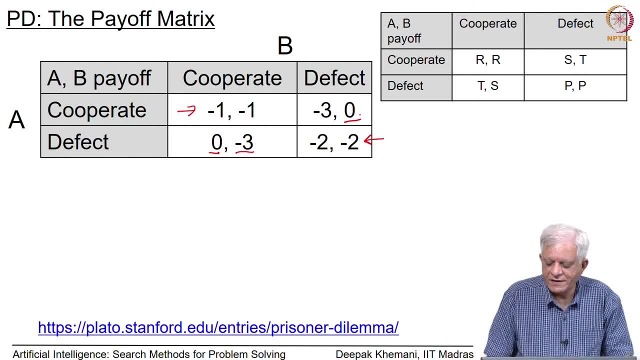 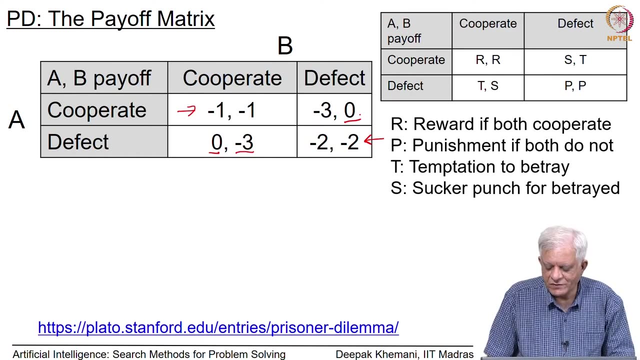 cooperate or they can defect, and the payoffs are R, R, S, T, T, S and P, P. The names are chosen such that R stands for reward if they both cooperate. So if they both cooperate, then they, they in some sense they both get let off lightly. P is the punishment if both do not. 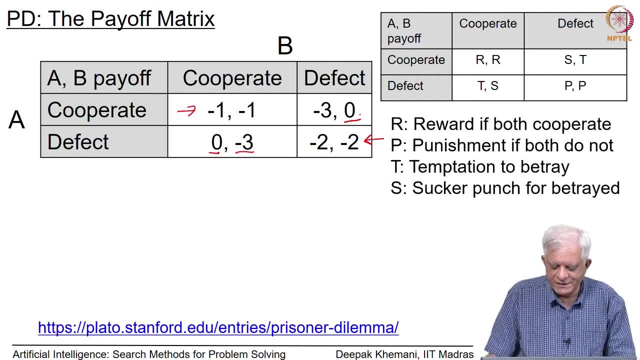 cooperate, betray each other, and both of them get punished. This is more than the punishment, is more than what they would have got if they had cooperated. T is a temptation to betray in which, of course, you get let off freely, and S is a sucker punch if you are, if you are the one who is betrayed. 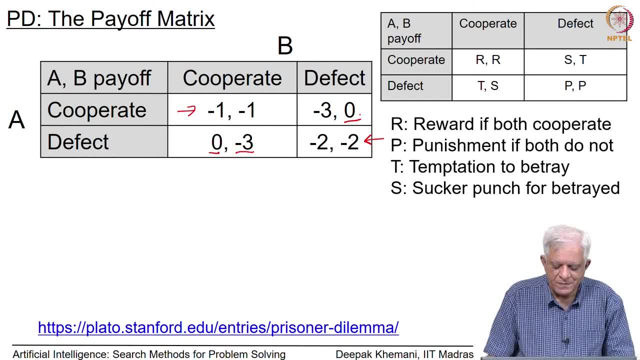 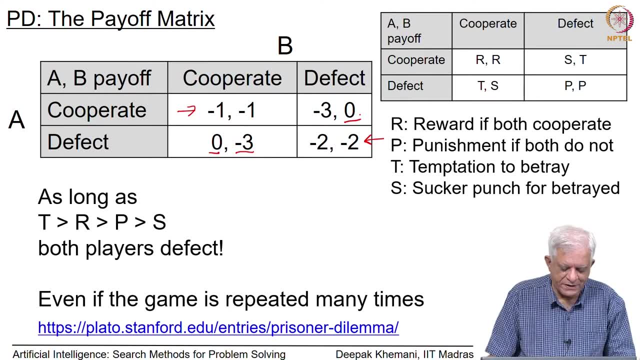 then that is the payoff that you get, And it has been shown and studied that, under the conditions that as long as T is greater than R and R is greater than P and P is greater than S- remember that T is the temptation of betraying- you get the maximum reward if you. 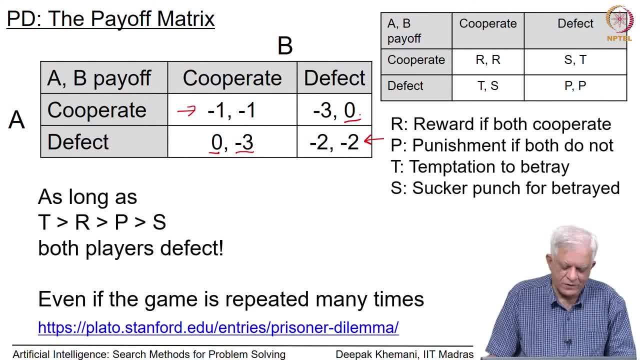 betray somebody: R is a reward if both of you cooperate, P is the punishment if both of you betray each other, and S is the reward that you get if you have been betrayed essentially Under these conditions, where T is greater than R and R is greater than P and P is greater 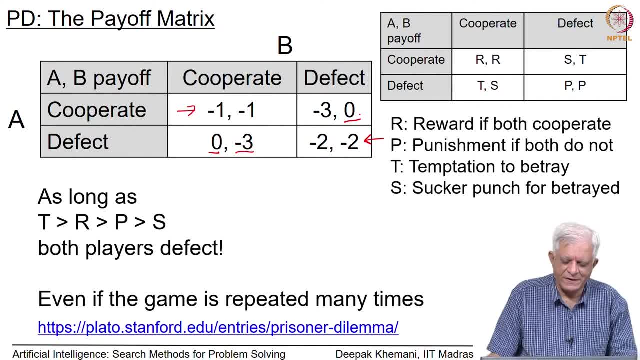 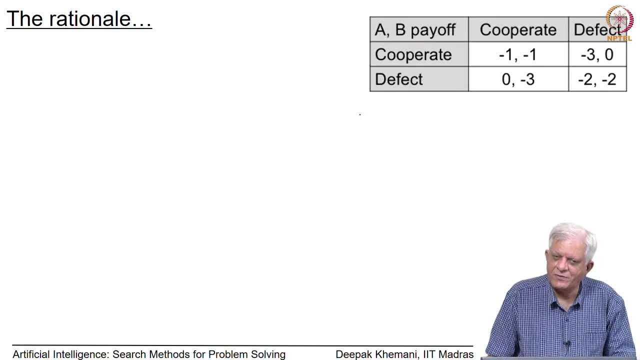 than S. it turns out that both players defect. It is rational for them to defect and they do so even if the game is repeated many times. that is the interesting part. Let us see why this is the case, So we can look at the rational. So remember that this is the payoff matrix that you have. 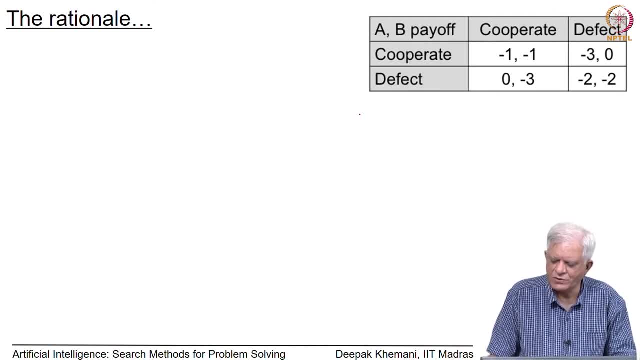 if you both cooperate, you get minus 1. if you both betray or defect, you get minus 2 each. if you betray the other, you get 0 and the other gets minus 3.. So let us see, I mean the game is actually happening simultaneously, in the sense that it is not a sequential game. 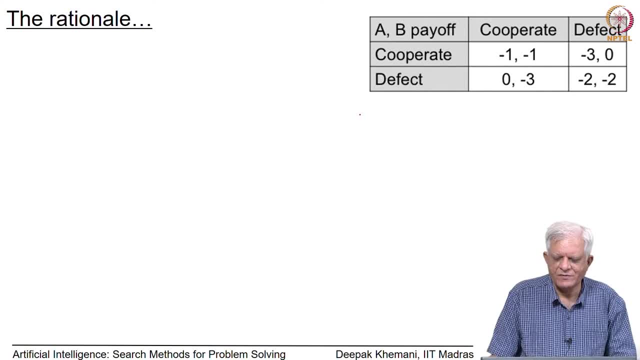 in which one player makes a move and then the other player makes a move, but we can think of the reasoning as a sequential process in which you can consider the various options of what the other player may be doing and what should be your strategy in that situation. 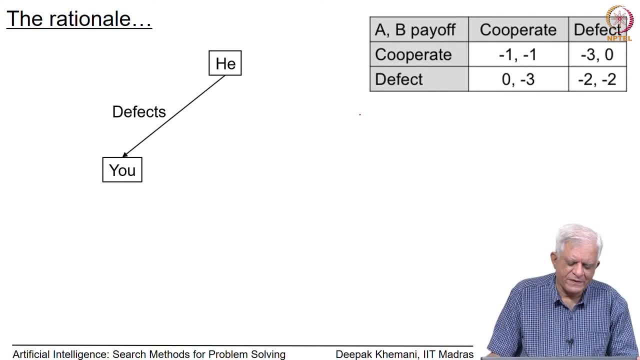 So we start up. So we start off by considering the situation where the other player betrays you or defects from defects from your team, so to speak. then what should you do? If you defect, you will get minus 2, as well as you can see from the table if, when both players defect, your payoff. 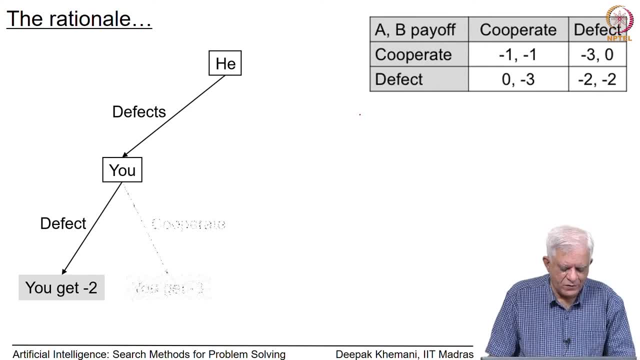 is minus 2.. If you cooperate with him, So he is betrayed, you and you are cooperating, then he will be let off with 0 and you will get minus 2.. So if you cooperate with him, So he is betrayed, you and you are cooperating, then he will be let off with 0 and you will 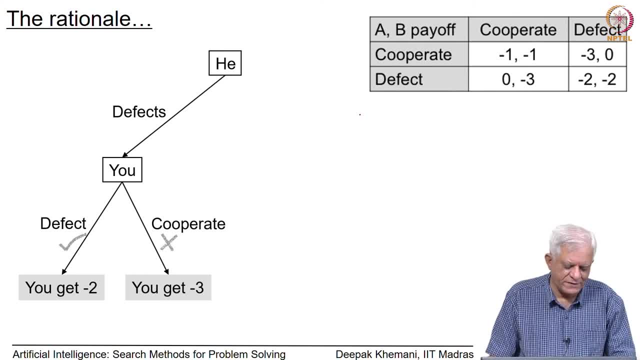 get minus 3.. So clearly, if he betrays or if he defects, then the correct choice for you is to also defect or to betray. essentially, Of course, you do not know whether he is betraying you or whether he is cooperating with you, but if he were to be betraying you, then your. 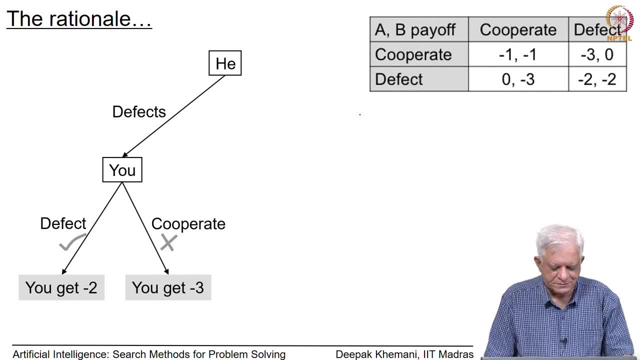 correct choice would be to also betray him. The other possibility is that he may cooperate with you. Now, if he cooperates with you, then you have those same two options. So you can say: if you defect, then you get let off from the prison without any sentence. So your 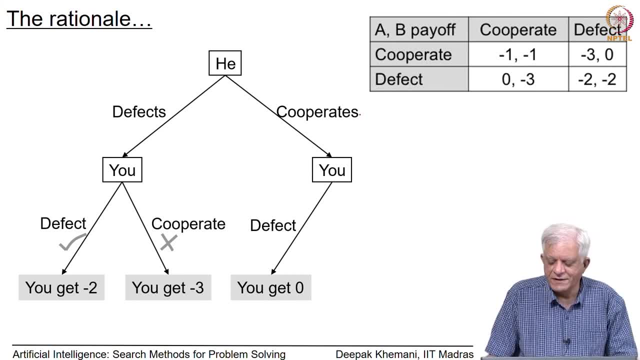 payoff is 0, which is the maximum payoff, incidentally, in this matrix, because the payoffs are negative and if you also cooperate, then both of you will get minus 1, a 1 year sentence in the prison. So clearly you can see that even in this scenario, for you to betray is the 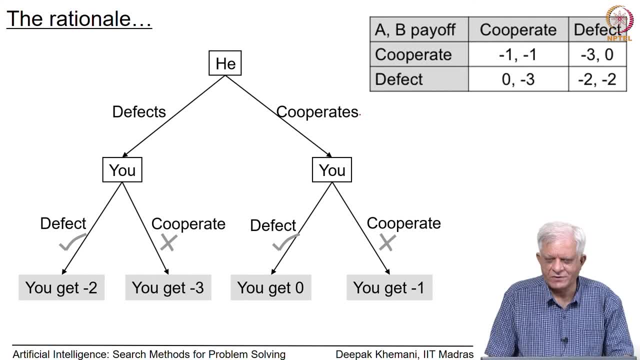 rational choice to make. So we are talking about rational choices. We are not talking about friendship and loyalty and other emotional parameters. We are simply talking of economic parameters in the sense that you just want to maximize your payoff and you can see that now why it is logical or rational to betray the partner if you simply want to maximize. 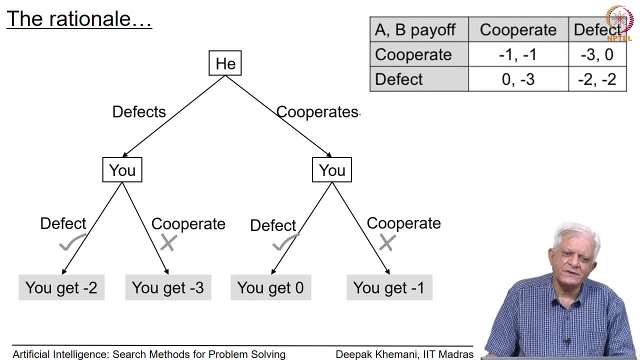 your payoff. So this shows that in many scenarios the Nash equilibrium that you reach is often not the optimal which sometimes people call as a Pareto optimal. In this case, the Pareto optimal would be when they both cooperate. If you sum up the total sentences that the 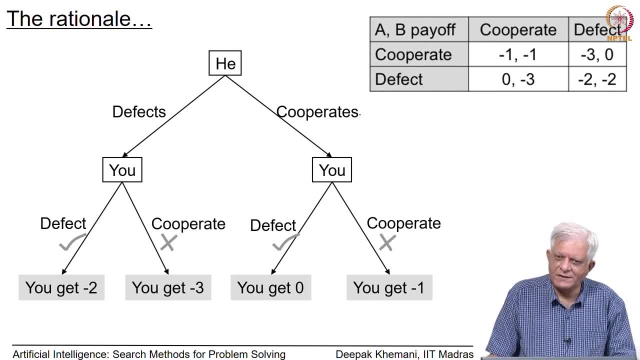 two players receive, then in the optimal, the total sentence is 2 years. in Nash equilibrium the total sentence is 3 years. So the Nash equilibrium that the two players receive is 4 years, but in the case of one betraying the other, the total sentences 3 years. ah, And you can see that the Nash equilibrium 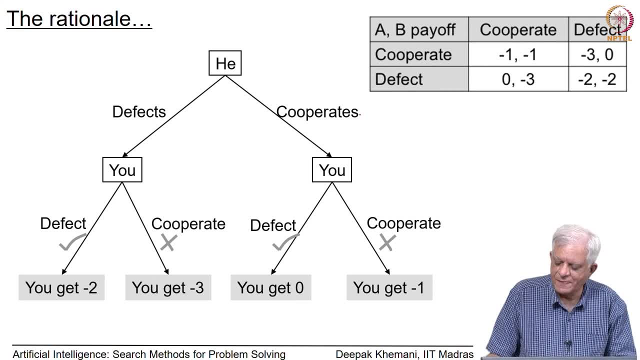 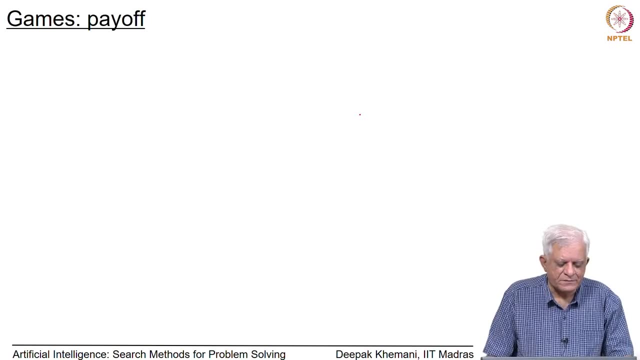 is settled into this ah lowest point, which is not the optimal point, where we both of you get 2 years into prison. Now let us quickly look at a classification of games before we move on. Games can be classified based on the payoff you get or the payoff that the different players get. The simplest of them is 0 sum games. 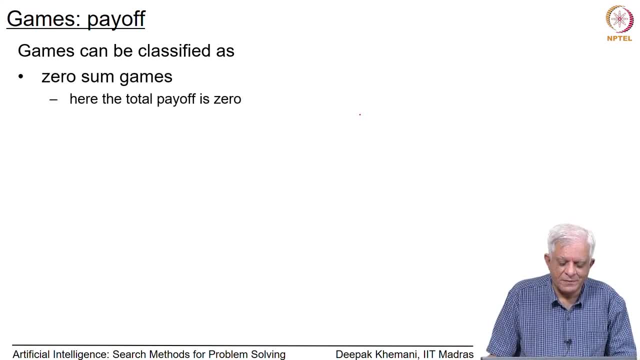 So in 0 sum games, the total payoff of all the players is 0. So which basically means that some players may gain, whereas at the cost of others, and the other players will lose. So this is typically a situation of competing for a payoff. it is typically a. 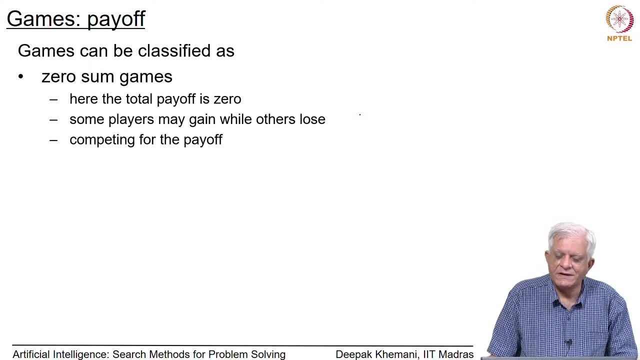 situation of pure competition or adversarial situation and any. most of the games that we play on the field, including things like football and so on, are situations which are 0 sum, that you win and the other side loses, and so on. But games do not have to be 0 sum, they can. 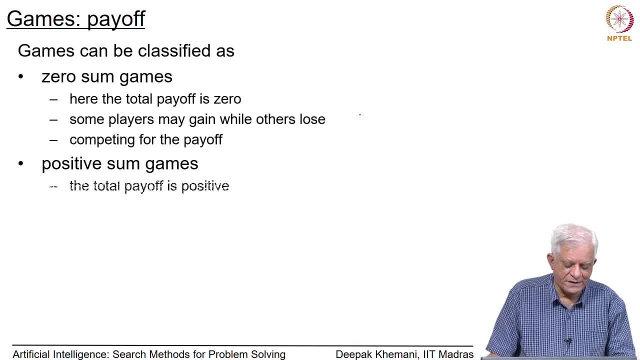 be positive sum games. these essentially model cooperation and the total payoff is positive. in this situation, most or all the players gain. So typical example of cooperation is, for example, when two students study together and help to clear each other doubts, then they can both benefit from it. or if two researchers 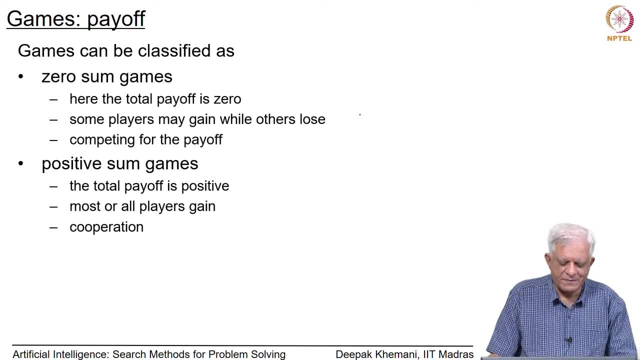 collaborate with each other, sharing methods and results, then both of them can benefit. So games can be positive sum games as well, but games can also be negative sum games where both the sides lose essentially. So the total sum, the total payoff here is negative and most of the players end up losing. 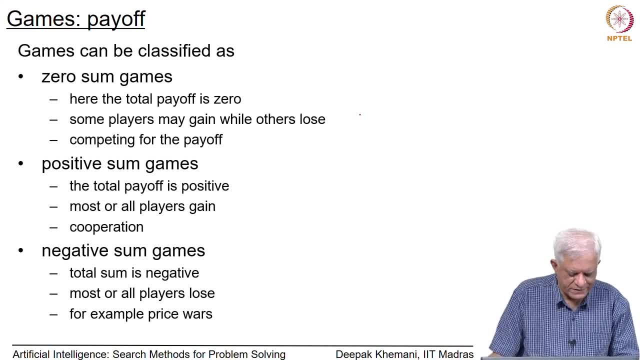 in the game. So environment is a situation like that, as you can imagine, but also simpler things like price power. if there are two companies which are selling a product and both of them try to gain market share by reducing the price of their product, then both of them end up. 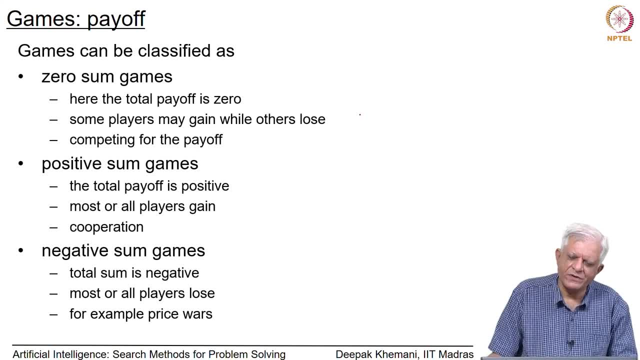 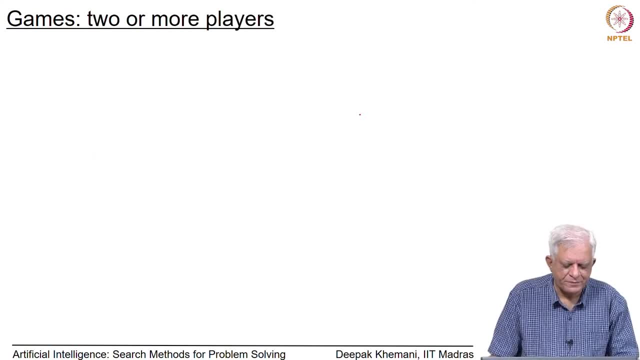 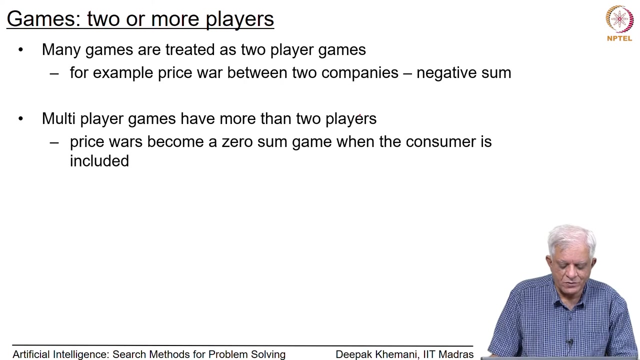 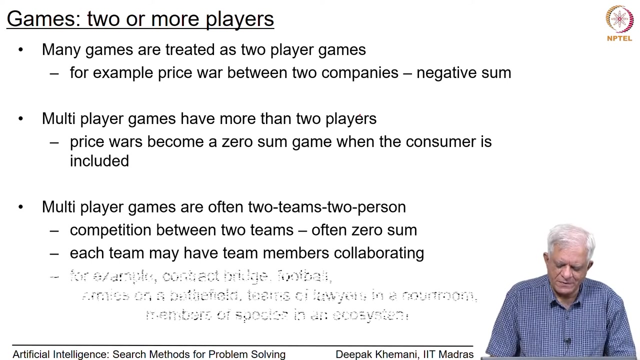 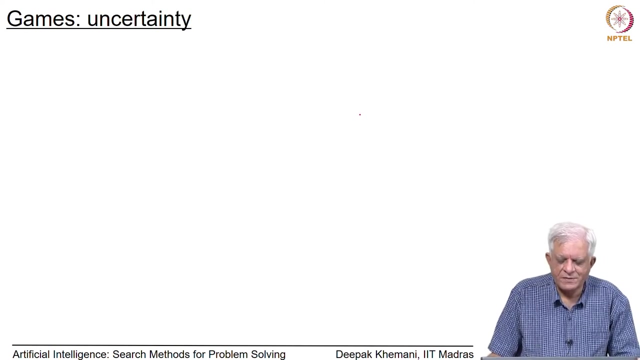 losing revenues. So that is why we looked at genetic algorithms. Games can also be model on how much information is available by amount of uncertainty in the situation. So incomplete information games lead to uncertainty. If you do not have enough information about those world, then clearly there is going. 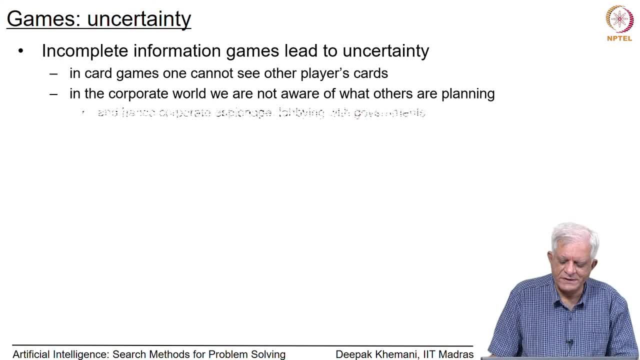 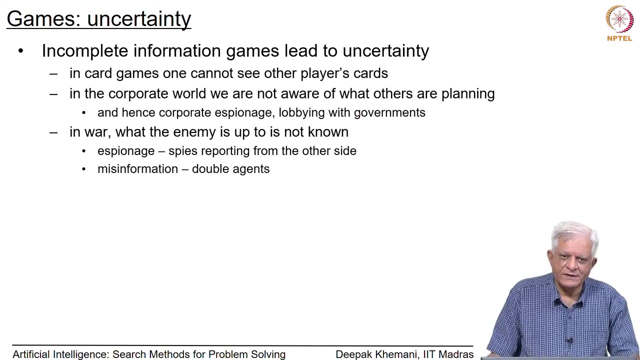 to be uncertainty and card games are typical examples, because you cannot see the other players cards. In the corporate world we are not aware of what other company's are. the companies are planning and very often you hear cases of corporate espionage or lobbying with governments to you know favor their own company. 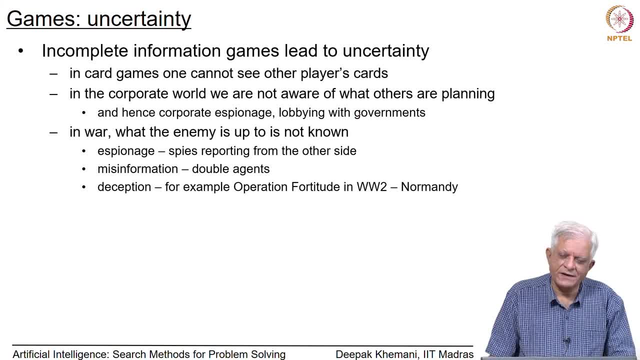 In a war like scenario, we do not know what the enemy is up to. again espionage spies reporting from the other side or use spreading misinformation via double agents. Information is a key part of incomplete information situations. For example, in the world war two, the allied forces, they fooled the Germans into thinking.